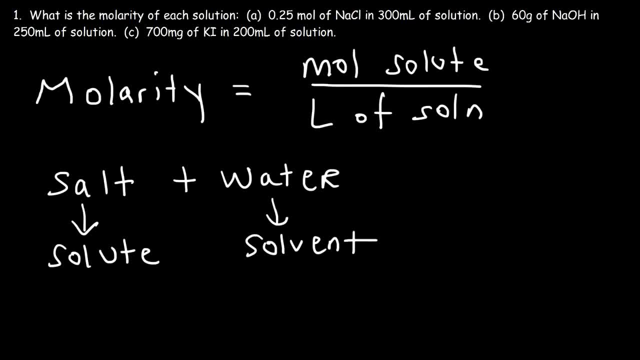 The solvent dissolves the solute And together the combination of the solute plus the solvent is the solution. So keep that in mind, So that will help you to distinguish the solute from the solvent. So now let's work on this example. 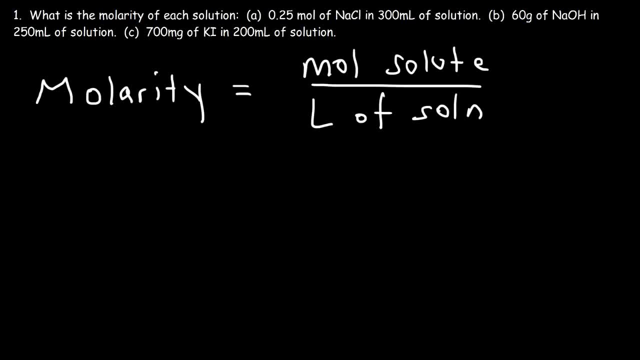 Let's focus on part A: 0.25 moles of sodium chloride in 300 milliliters of solution. What is the molarity of that solution? So we're given everything that we need. We have the moles of the solute. 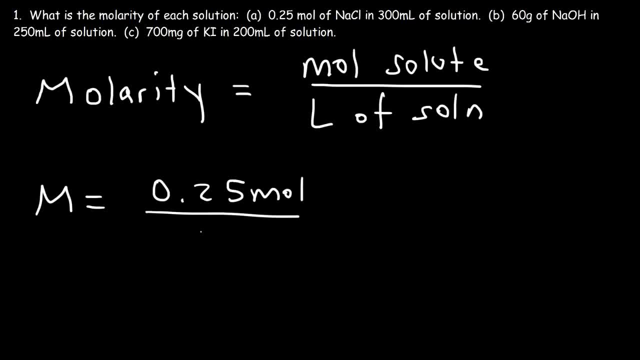 Sodium chloride dissolves in the solution And we have the volume of the solution. However, we need to convert it to the unit's liters. And to convert milliliters to liters, simply divide by 1,000.. One liter is equal to 1,000 milliliters. 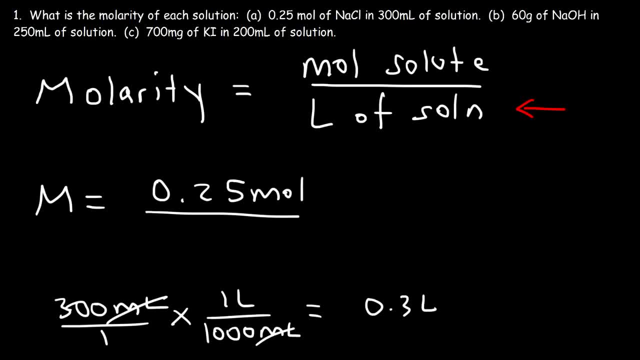 So 300 divided by 1,000, it's 0.3.. Another thing that you can do is move the decimal three units to the left. So let's divide this by 0.3 liters And 0.25 divided by 0.3.. 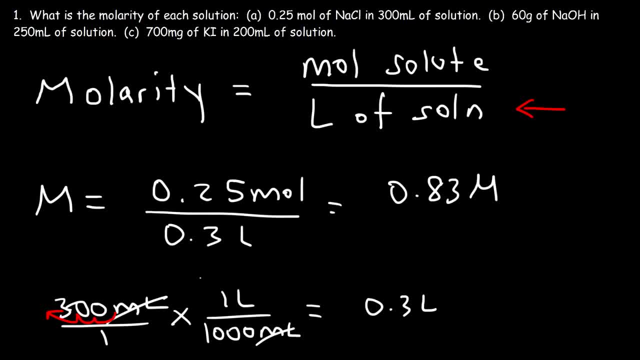 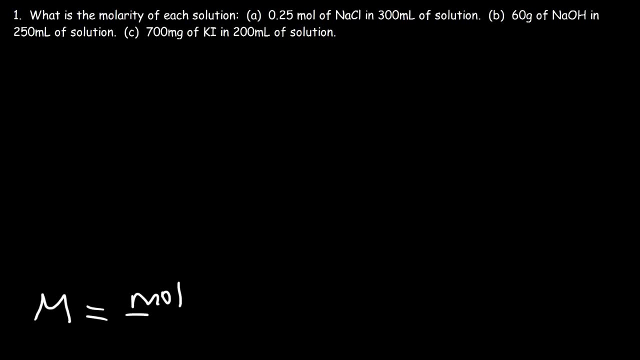 That's about 0.83.. So that's the concentration of the first solution in part A. Now let's move on to part B. Now keep this in mind: Molarity is moles of solute divided by liters of solution. This will be helpful throughout parts B and C. 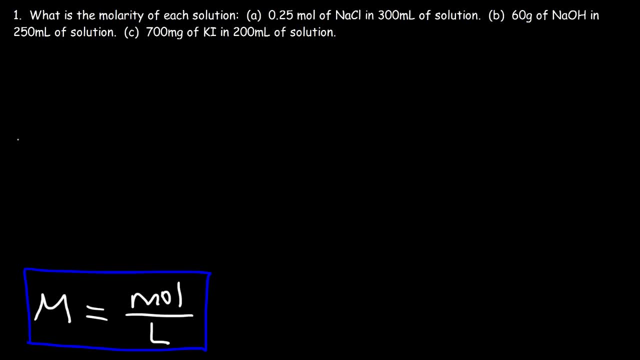 So for part B I'm going to do more of a conversion process. Let's start with 60 grams of sodium hydroxide. Now I need to get moles. I want to have the unit moles on top and on the bottom the unit liters. 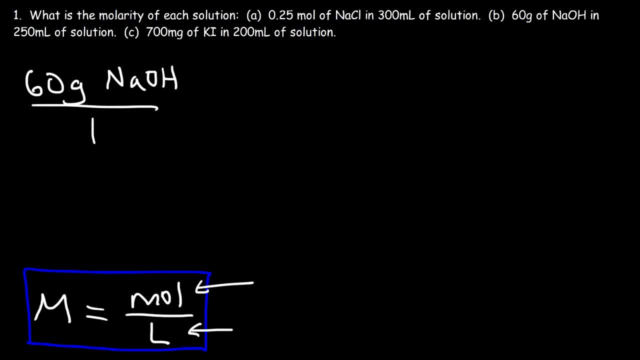 So let's convert grams to moles And we need to find the molar mass of sodium hydroxide to do that. So we need to add up the atomic mass of sodium, oxygen and hydrogen, So sodium is about 22.99.. 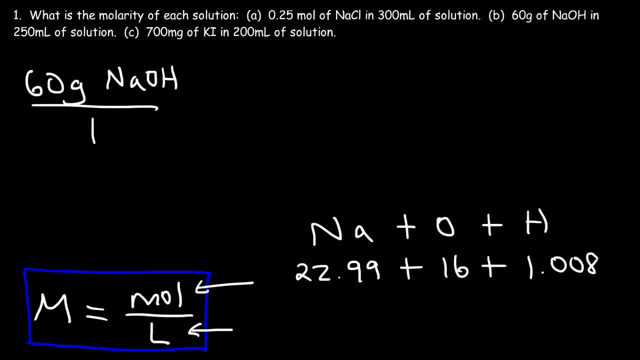 Oxygen is 16.. Hydrogen is 1.9.. Hydrogen is 0.008.. So this is 39.998.. But for all practical purposes let's round it to 40.. So we can say that one mole of sodium hydroxide has a mass of 40 grams. 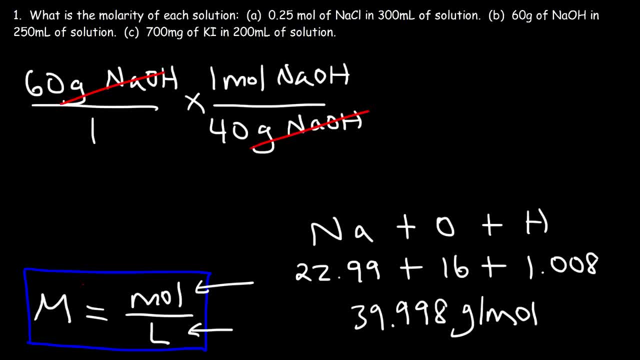 So now we no longer have the unit grams of sodium hydroxide. Now all we need to do is take the moles And divide it by the liters. But we need to convert 250 milliliters to liters. So if you take 250 and divide it by 1,000, you'll get the volume in liters, which is 0.25 liters. 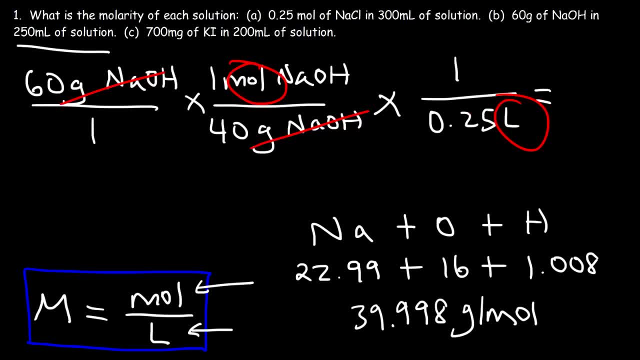 So notice that we have the unit moles on top and liters on the bottom. Whenever you have that, your answer is the concentration in molarity. So it's 60 divided by 40.. And then take that result, divide it by 0.25.. 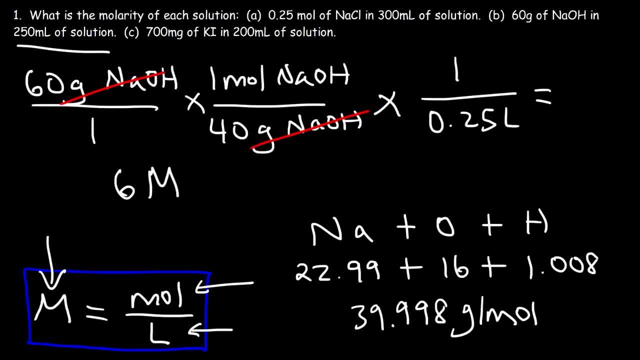 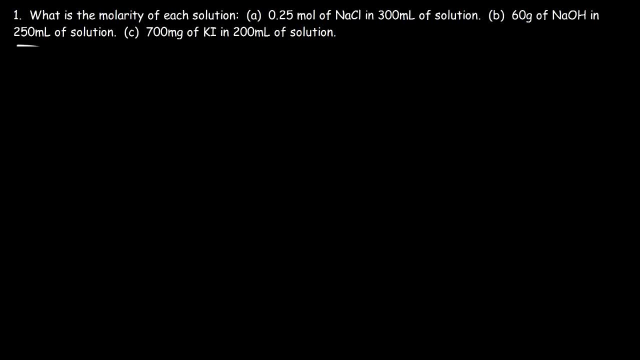 0.25.. So the concentration is 6 molar Or 6 moles per liter. So that's the answer for part B. Part C, Let's find the molarity of the solution when 700 milligrams of potassium iodide is dissolved in 200 milliliters of solution. 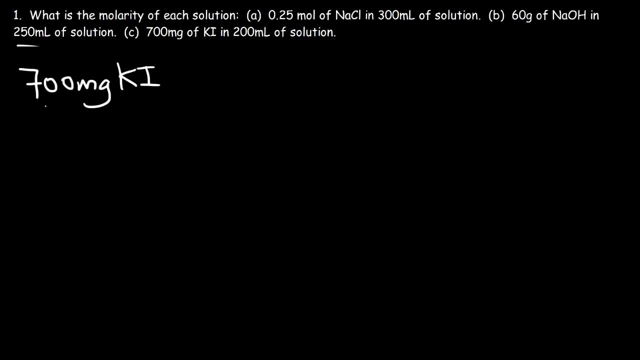 So let's start with what we're given. Now we need to convert milligrams to grams, and then grams to moles, And then take the number of moles divided by the liters. One gram is equal to 1,000 milligrams. 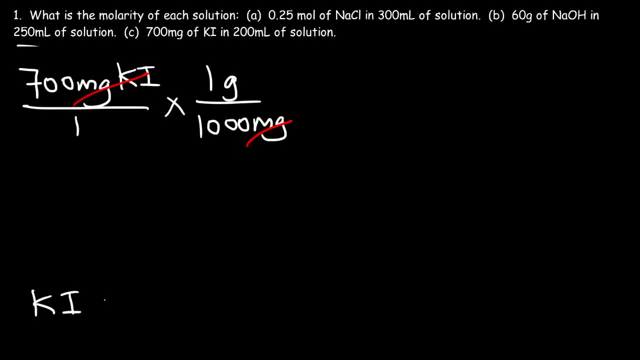 And now we need the molar mass of Ki. The atomic mass of potassium is 39.1.. And the atomic mass of iodine is 120.. So the total is 126.9.. So the sum is 166 grams per mole. 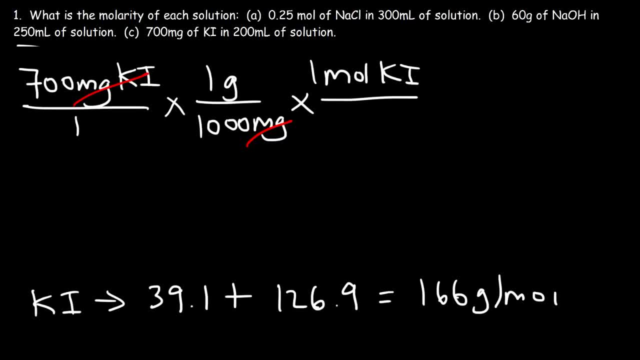 So one mole of Ki has a mass of 166 grams. Now the last thing we need to do is take the moles divided by the number of liters in the solution, So 200 milliliters If you divide that by 1,000. 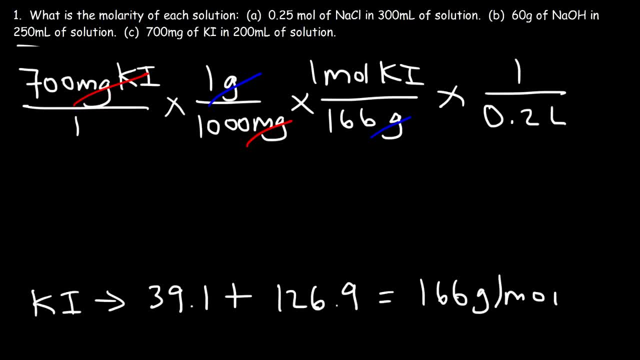 That's 1,000.. Then you have 1,000.. That's 0.2 liters, and so that's going to give us the answer. So it's 700 divided by 1,000, divided by 166, divided by 0.2.. 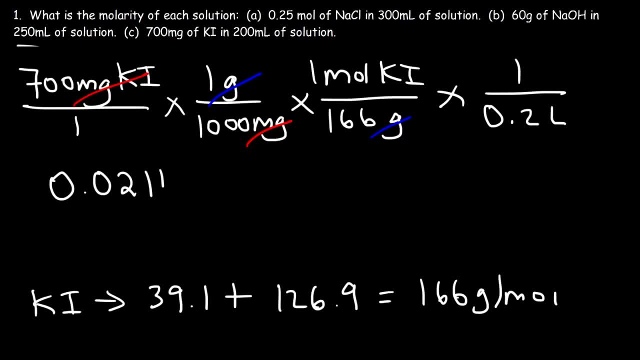 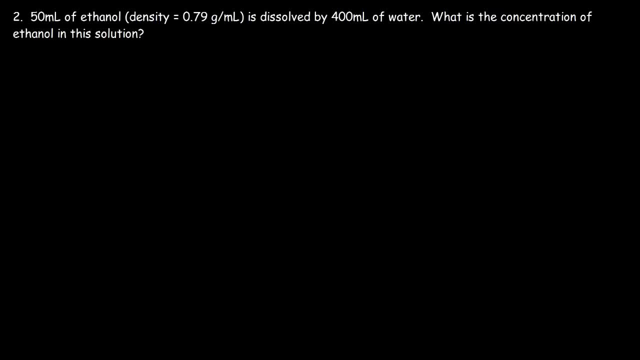 So the concentration is 0.0211.. So that's the molarity of the potassium iodide solution Number two: 50 milliliters of ethanol is dissolved by 400 milliliters of water. What is the concentration of ethanol in this solution? 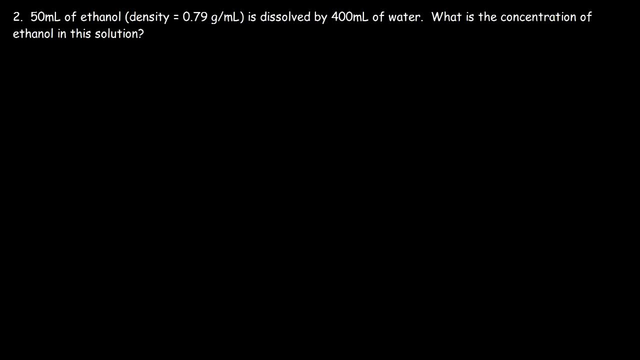 So which one is the solute and which one is the solvent? The solute is dissolved by the solvent. The solvent is water. in this problem, The solute is ethanol. Typically, the solvent is usually in greater quantity than the solute. 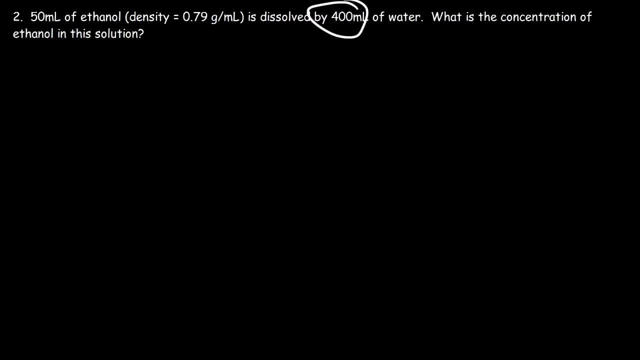 We have a lot more water than ethanol, so water dissolves ethanol in this case. Now, in order to find the concentration, we'll need to calculate the moles of the solute, So we've got to get the moles of ethanol. 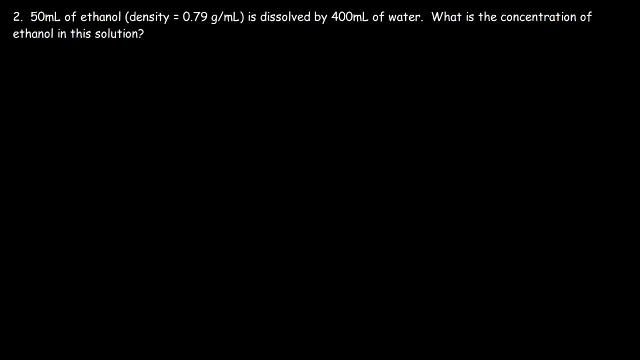 and then divide it by the liters of the solution. Now, if you recall, the solute plus the solvent combined makes up the solution. So what is the volume of the solution? We have 50 milliliters of solute, 400 milliliters of solvent. 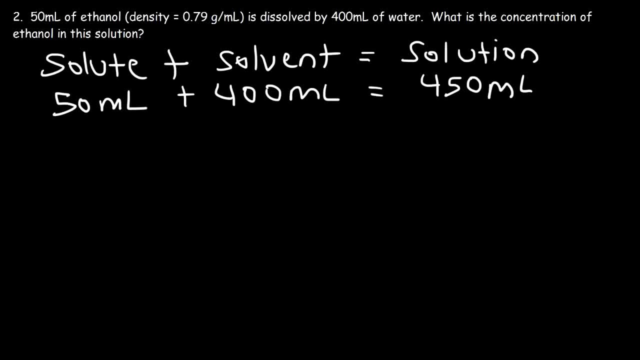 So therefore, we have 450 milliliters of solution, And if you divide that by 1,000, that's 0.45 liters of solution. So we're going to use that later. So now we need to focus on finding. 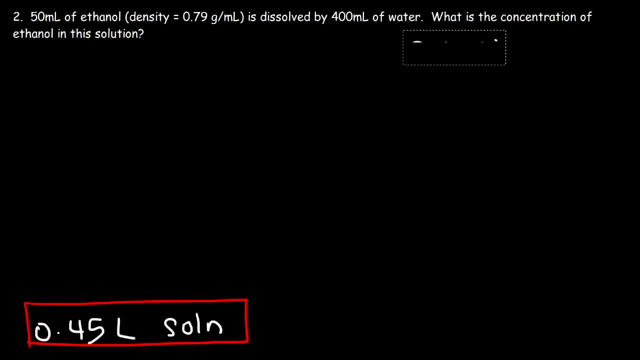 the moles of the solute, which in this case is ethanol. So we have the volume and we have the density Combined. we can use that to get the grams of ethanol and then convert that into moles. By the way, here's the formula for ethanol. 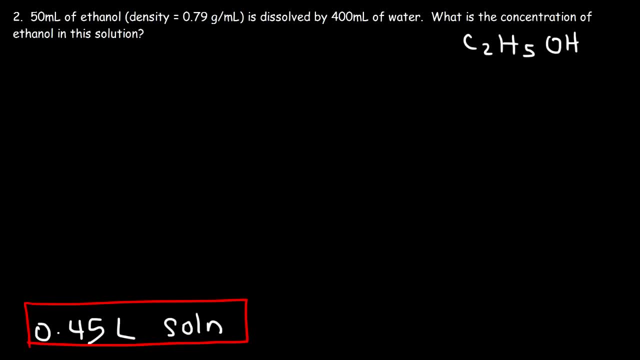 C2H5OH, So you can always look that up on the internet or something. So let's start with the volume of ethanol. We have 50 milliliters of ethanol and the density of ethanol is 0.79 grams per milliliter. 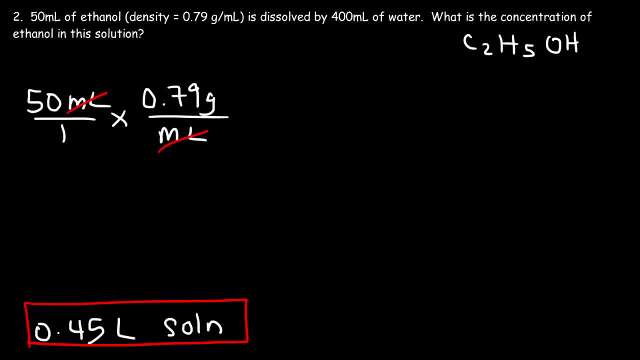 So now we have the mass of ethanol in grams, So now we can convert that to moles. but we've got to find the molar mass. So ethanol contains two carbon atoms, six hydrogen atoms and one oxygen atom And a single molecule. 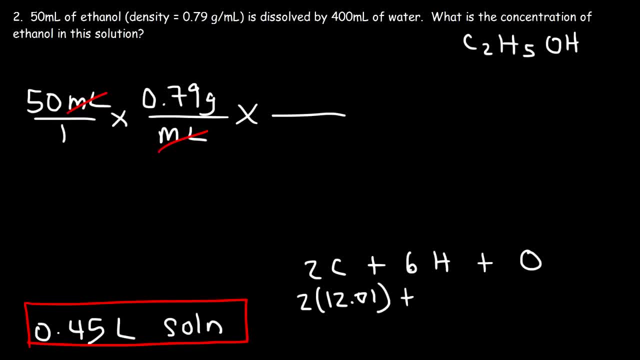 So this is 2 times 12.01 plus 6 times 1.008 plus 16.. So this adds up to 46.068 grams per mole. So that's the molar mass, That's the density of ethanol. So one mole is equal to 46.068 grams. 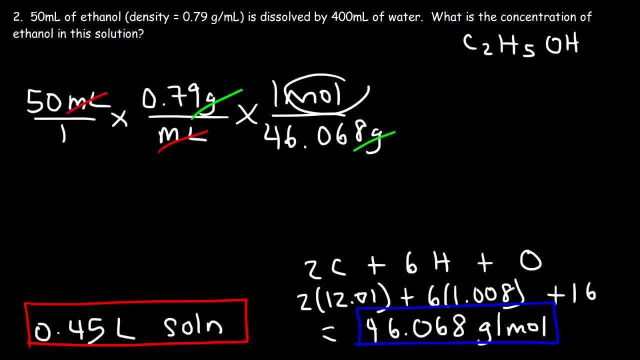 Now the last thing we need to do, once we have moles, is to divide by the number of liters, which we know it's 0.45.. So once you have these two units, moles divided by liters, you now have the molarity of the solution. 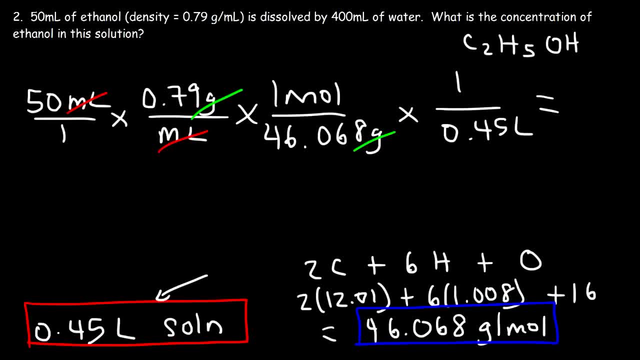 So it's 50 times 0.79 divided by 46.068, and then take that result divided by 0.45.. So the concentration is 1.905.. So that's the molarity of the solution Number three. 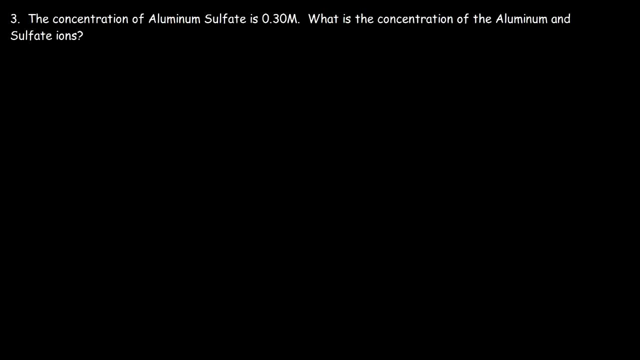 the concentration of aluminum sulfate is 0.3 moles per liter. What is the concentration of the aluminum and sulfate ions? Well, first let's write the chemical formula of aluminum sulfate. Aluminum is found in group 3A of the periodic table. 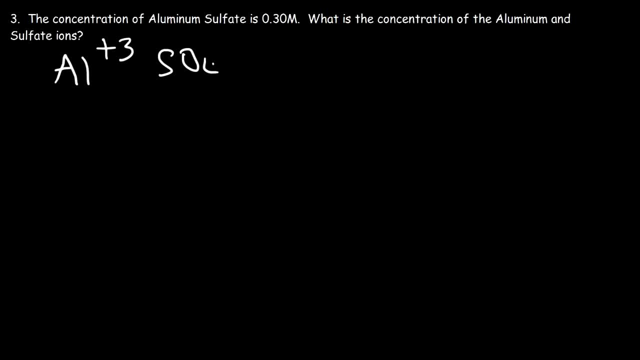 So it has a positive three charge, And sulfate is one of those polyatomic ions that you should know by now. It's SO4 2-, And so the chemical formula is gonna be Al2SO4 3. And the concentration is 0.30 moles per liter. 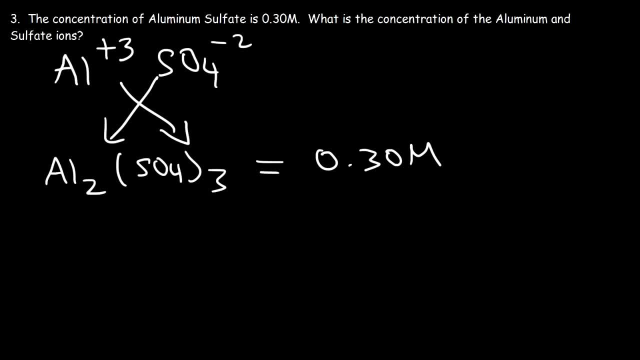 And the concentration is 0.30 moles per liter. And the concentration is 0.30 moles per liter. So, based on that, what is the concentration of the aluminum plus three cation? So notice that we have a subscript of two. 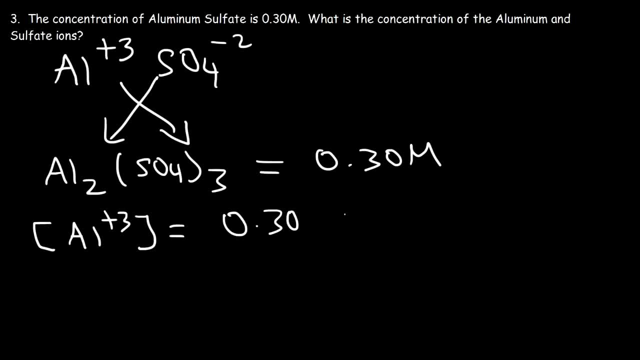 So it turns out that to find it, all you gotta do is multiply the molarity by two, So it's gonna be 0.60.. And in the case of sulfate, there's three of them per formula unit, So it's gonna be 0.60.. 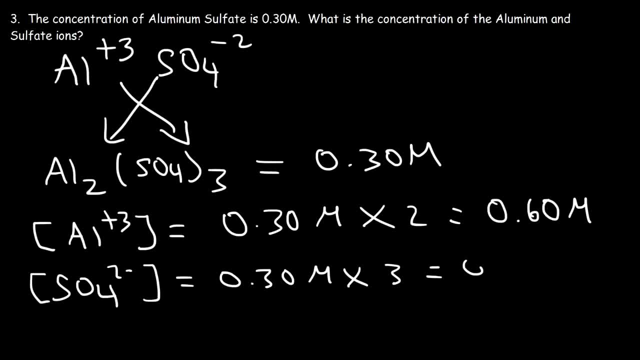 And in the case of sulfate, there's three of them per formula unit. So it's gonna be 0.30 times three, which is 0.90.. which is 0.90.. Now for those of you who need to show your work. 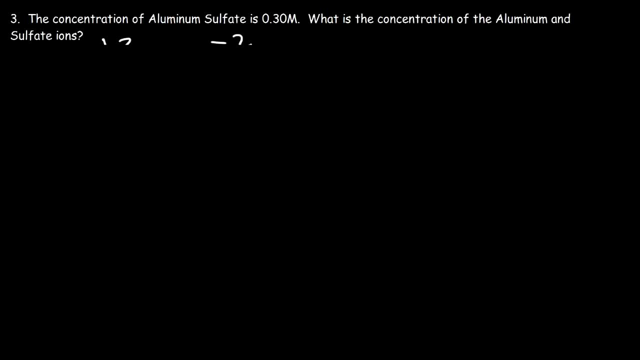 here's what you can do. here's what you can do. The first thing you should do is write the dissolution of aluminum sulfate. Aluminum sulfate breaks down into two aluminum cations. Aluminum sulfate breaks down into two aluminum cations And three sulfate ions. 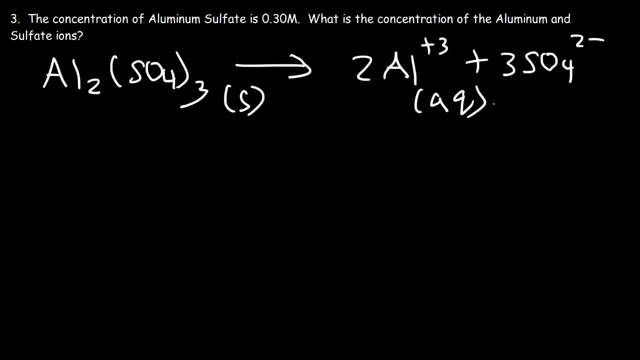 So you could say this is the solid phase and, on the right, the aqueous phase. So I'm gonna represent this as 0.3 moles of aluminum sulfate per liter, because that's what it is. Molarity is moles per liter. 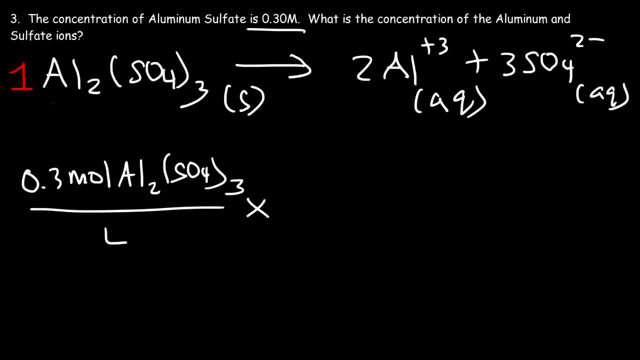 Now we can use the molar ratio. Now we can use the molar ratio to convert from- I'm gonna use sulfate as an example- So from aluminum sulfate to sulfate it's a one to three ratio. So for every one mole of aluminum sulfate that dissolves, 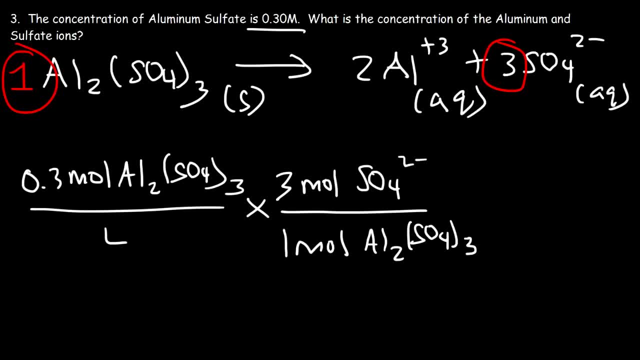 three moles of sulfate ions are released into the solution, So the unit moles of aluminum sulfate will cancel. So now what you have left over is moles of sulfate per liter of solution, So it's 0.3 times three. 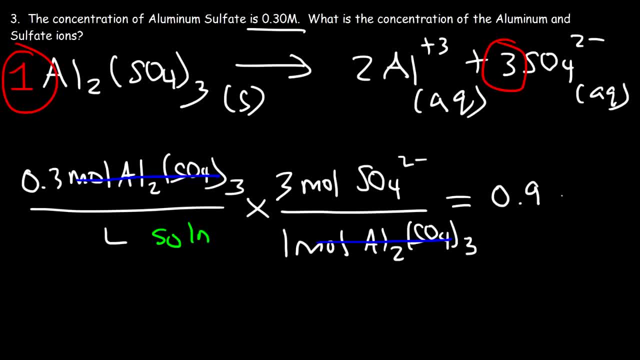 And so this will give you 0.9 moles per liter, which you could say that's 0.9 molar sulfate. So that's the concentration of sulfate. That's how you can show your work, if you want to. 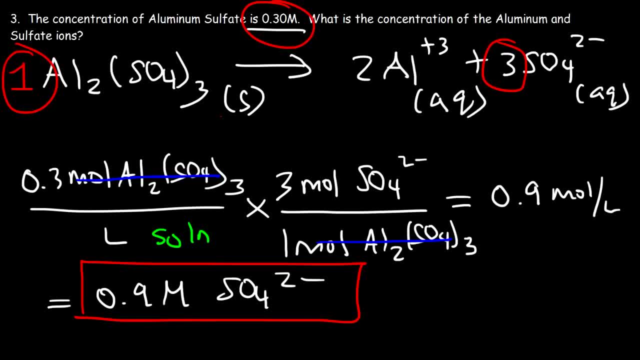 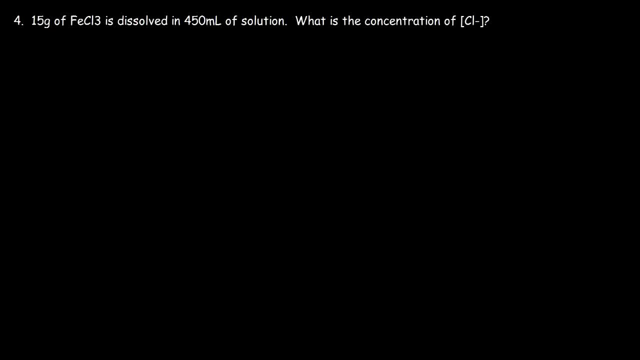 But the simplest way to get the answer is to take 0.3 and multiply by the subscript And that will give you 0.9.. Number four: 15 grams of iron chloride is dissolved in 450 mL of solution. What is the concentration of chloride? 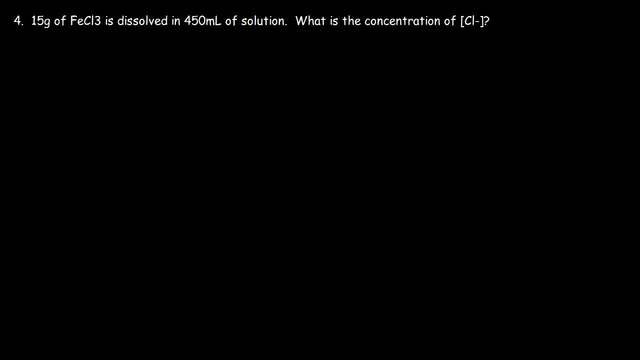 So let's get the answer just completely using conversions and dimensional analysis. Let's start with 15 grams of FeCl3.. Now, in order to get the concentration, we need to convert this into moles And at the same time, we need to change the substance from FeCl3 to Cl-. 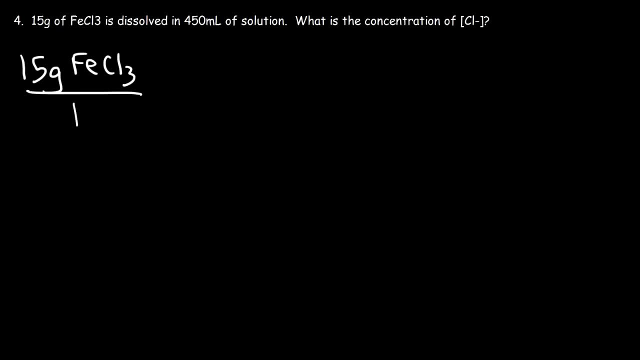 So that's going to require an extra step. But first let's calculate the molar mass of FeCl3.. So we have one iron atom and three chlorine atoms. The atomic mass of Fe is 55.85.. And the atomic mass of Cl is 35.85.. 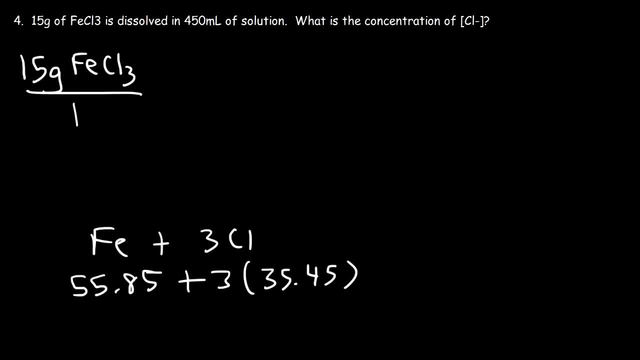 So you should get a molar mass of 162.2 grams per mole. So one mole of FeCl3 has a mass of 162.2 grams. So that's going to require an extra step. So let's get the answer just completely using conversions and dimensional analysis. 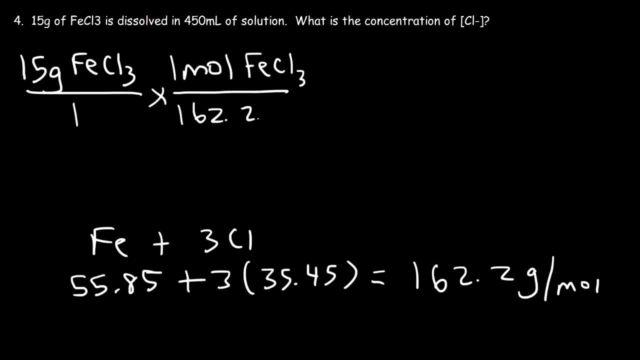 What is the concentration of FeCl3?? What is the concentration of FeCl3?? The atomic mass of FeCl3 is 55.85.. And the molecular mass of FeCl3 is 52.52 grams. So let's look at it now. 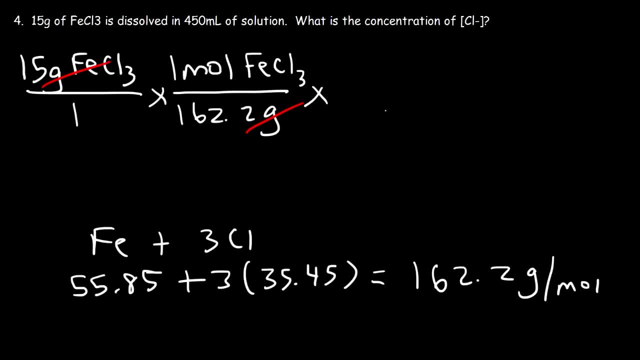 Now the reaction to this point is a little stuffy, And here's the reason: If we have如果你 and you have Berkeley, Now they have a mixture of충les, a changing mixture of dingen with chlorine and chlorine. Applause. 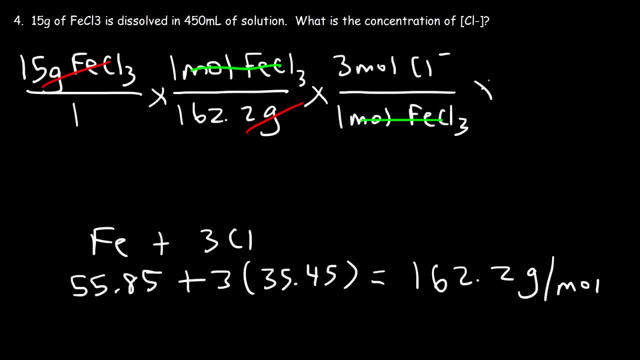 moles of chloride ions. all we need to do is divide it by the liters of solution and that will give us the concentration of chloride. So let's divide this by 1000 to convert it to liters, So that's 0.45 liters. 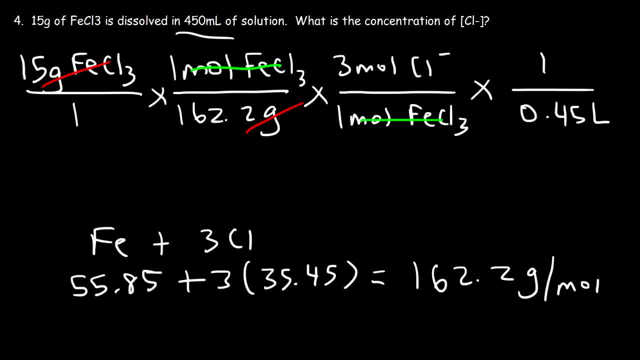 So this is going to be 15 divided by 162.2 times 3 divided by 0.45.. So the concentration of chloride in a solution is 0.617 moles per liter or capital M. So that's the molarity of the solution of the chloride in a solution. 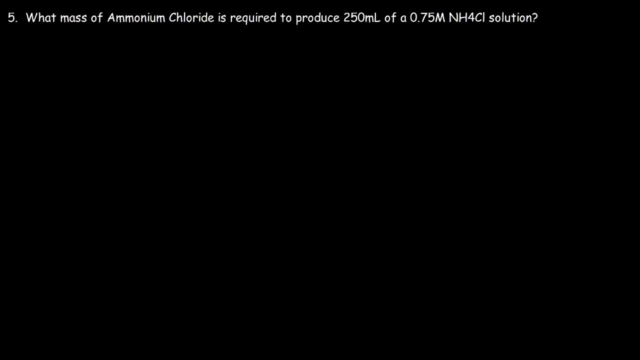 Number five: what mass of ammonium chloride is required to produce 250 milliliters of a 0.75 molar ammonium chloride solution? So we're going to do this. So we're going to do this. So we're going to do this. 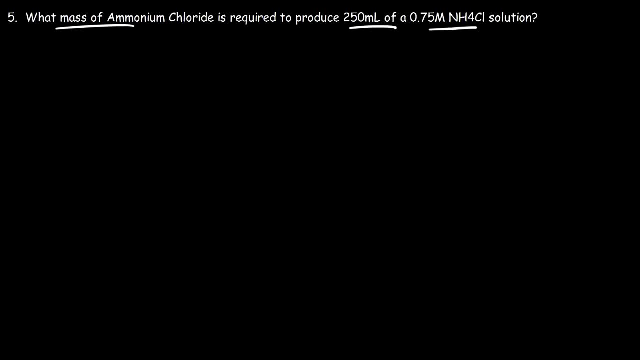 So, given the molarity and the volume, how can we find the mass? The best way is to convert it. I'm going to start with the molarity of the solution. So keep in mind capital M molarity. you can represent it as moles per liter. 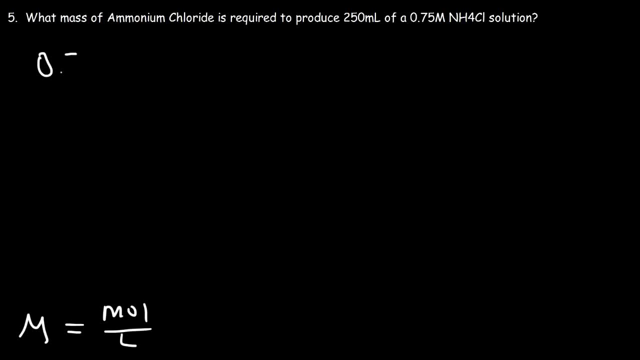 So a 0.75 molar solution means that we have 0.75 moles of ammonium chloride per liter of solution. Now we're not going to change the substance, so we don't need to write NH4Cl. So I'm just going to write this 0.75 moles per liter. 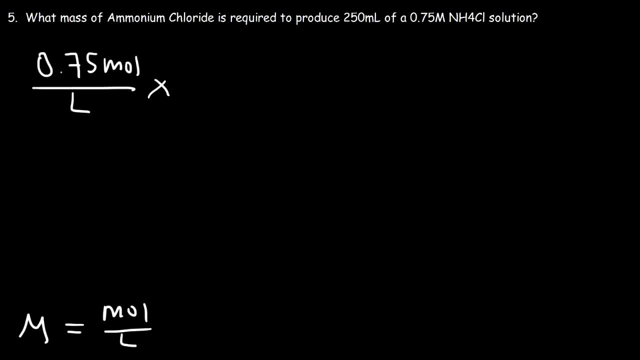 Now we have the volume of the solution: 250 milliliters, and if we divide that by 1000, that's 0.25 liters. You want to multiply the molarity by the volume because if you noticed the unit liters will. 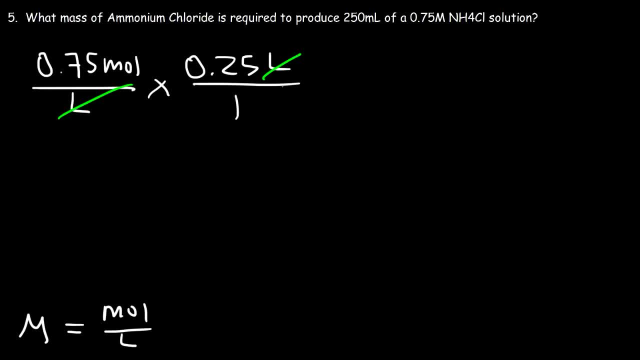 cancel, and now we have the moles of ammonium chloride. So all we got to do is change moles to grams, and we can do that using the molar mass. So in NH4Cl. In NH4Cl we have one nitrogen atom, four hydrogen atoms and a Cl atom. 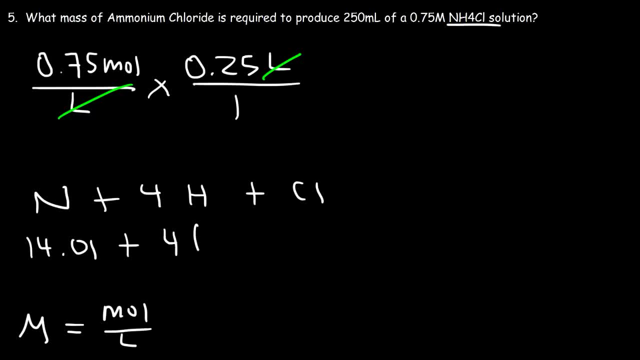 Nitrogen is 14.01,, H is 1.008, and Cl is 35.45.. So the molar mass is 53.492.. Now, because we have the unit moles on the top left, we need to put the moles on the bottom. 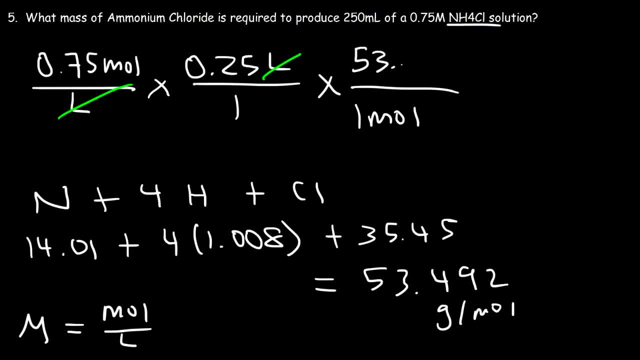 So one mole of NH4Cl has a mass of 53.45.. So this is going to be 0.75 times 0.25 times 53.492.. So the answer that I got is 10.03 grams of NH4Cl. 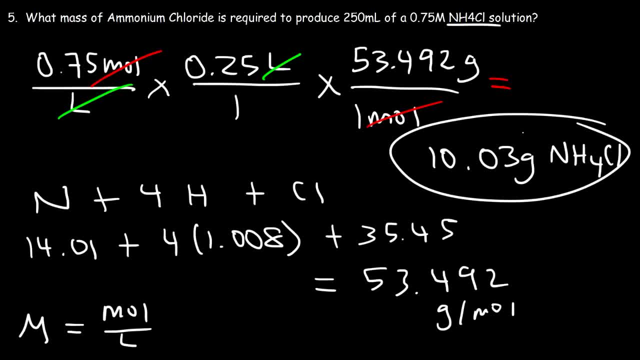 So if you're given the volume and the molarity and you want to find the mass, you need to take the molarity and multiply it by the volume in liters And then multiply it by the molar mass of the substance. That's going to give you the grams of the substance. 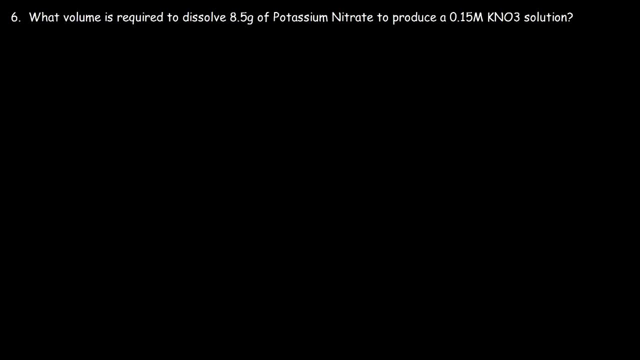 Number six: what volume is required to dissolve 8.5 grams of potassium nitrate to produce a 0.15 molar potassium nitrate solution? So this time we're given the mass of the solute, the molarity of the solution. 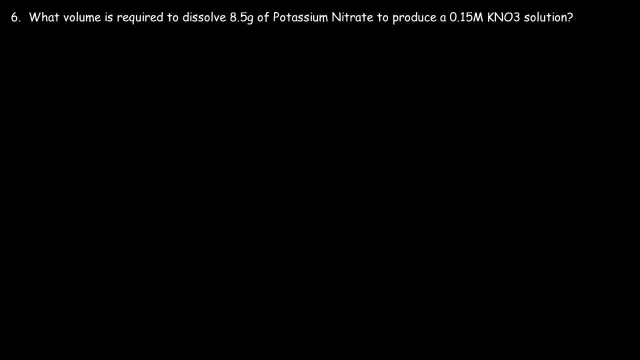 and our goal is to find the volume. We're going to find the volume first in liters And then we're going to convert it to milliliters. So how should we begin Now? if we want to get liters on top, that means molarity has to be on the bottom. 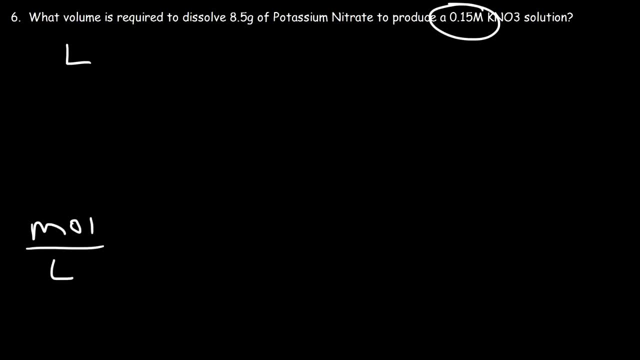 We don't want to start with molarity, because that's going to be moles per liter. However, we need to flip it at some point because we want this unit to be on top. Just keep that in mind. So let's start with the mass. 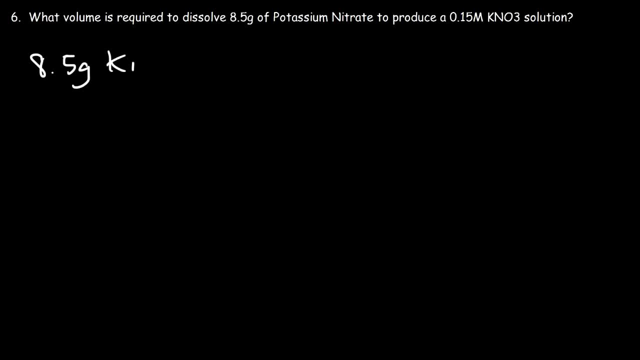 So 8.5 grams of KNO3.. And here's the basic setup that I'm going to do. I'm going to start with the grams And then, using the molar mass of the substance, this will give me the moles. 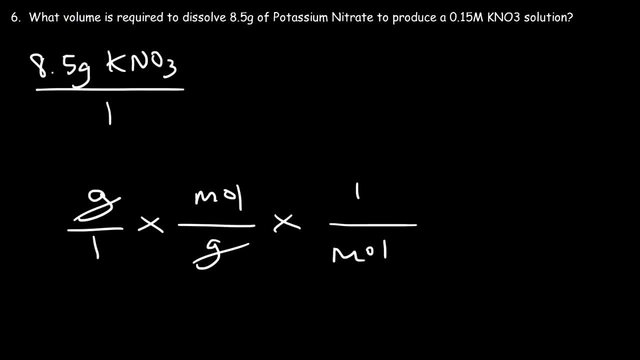 And using the molarity, I'm going to get the liters on top, which is what I want. So that's just a blueprint of how I'm going to set up the conversion process, And I don't like when the whole thing just disappears like that. 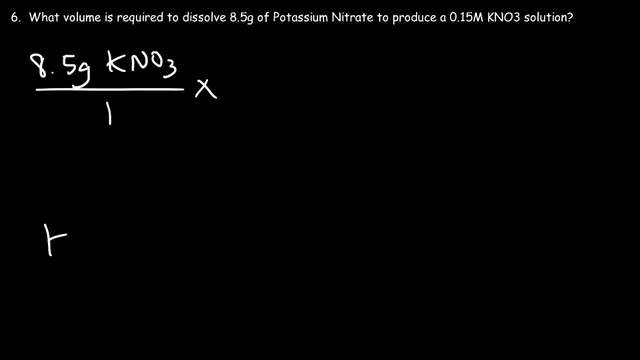 So we need to find the molar mass of KNO3.. Potassium has an atomic mass of 39.1.. N is 14.01.. And O is 16.. 3 times 16, that's 48..